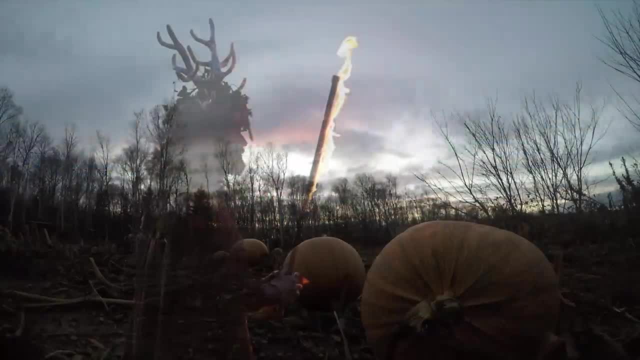 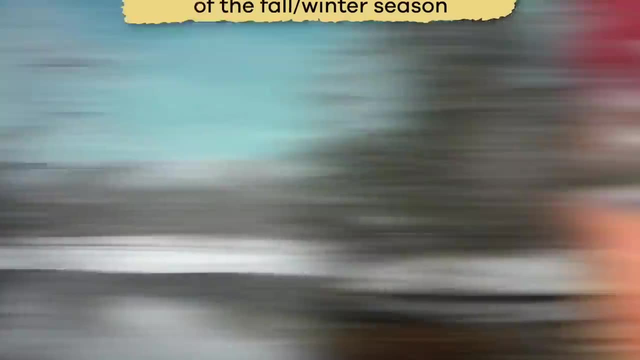 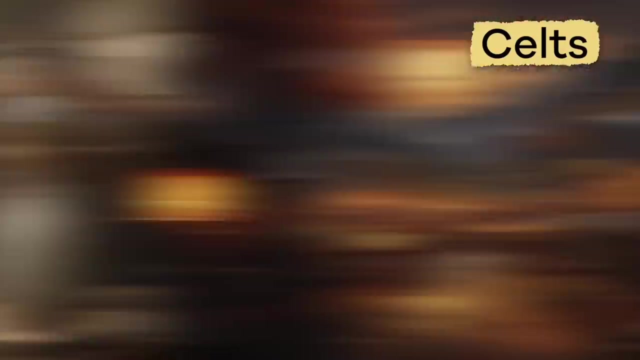 It's true. It began centuries ago as a way to mark the transition between the end of summer and the beginning of the fall-winter season. That is why Halloween is celebrated in the fall. Historians believe that Halloween originated with the Celts. 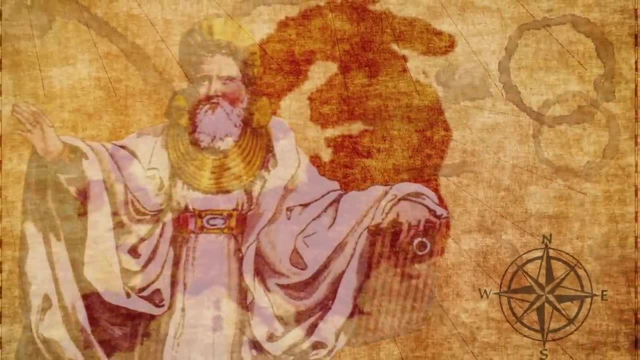 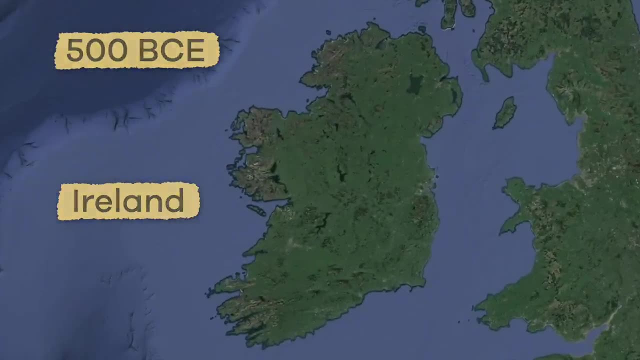 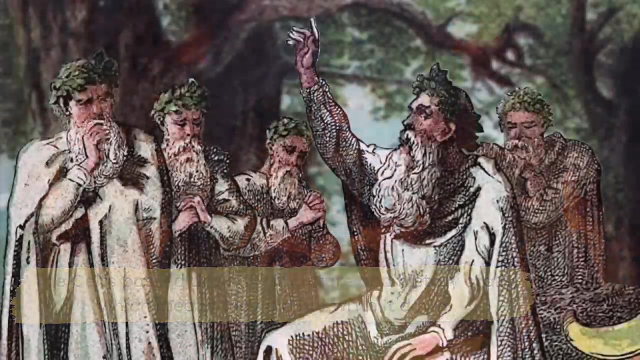 The Celts were once the largest geographical group to live in ancient Europe, before they settled in what is now Ireland. around the year 500 BCE, The Celts passed down their culture and history orally, which means they did not write it down. Celtic priests called Druids were responsible for passing all Celtic traditions on to the next generation. The Celts thought that when a person died, they transitioned or changed from physically living on Earth to living in a spiritual world. Because of this belief, they would celebrate the burial of their dead with feasts and parties. They also celebrated the new year with a festival called Sowin, which can also be pronounced Sow-in. 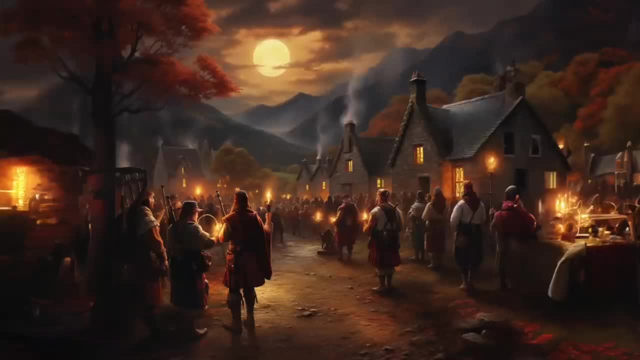 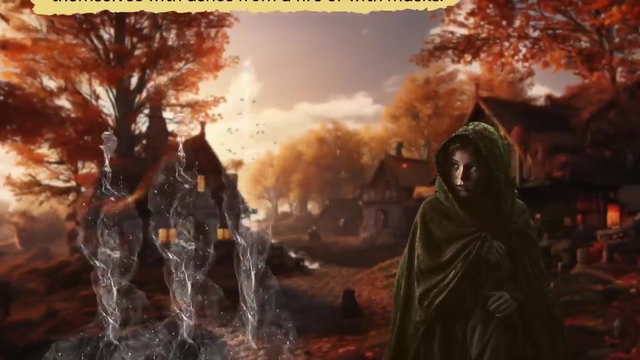 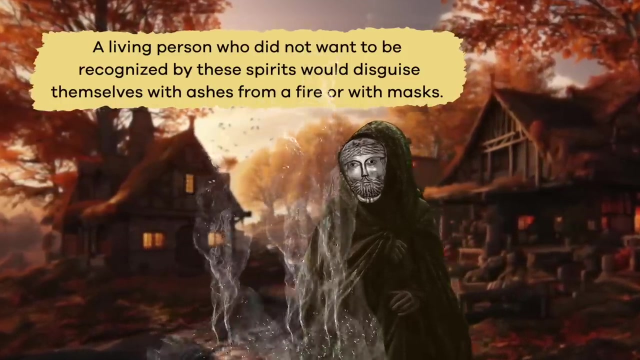 The Celts would stock up on supplies for the coming winter and welcome guests from the afterlife. Sometimes, unwanted or evil spirits would appear and a living person who did not want to be recognized by these spirits would disguise themselves with ashes from a fire or with masks. 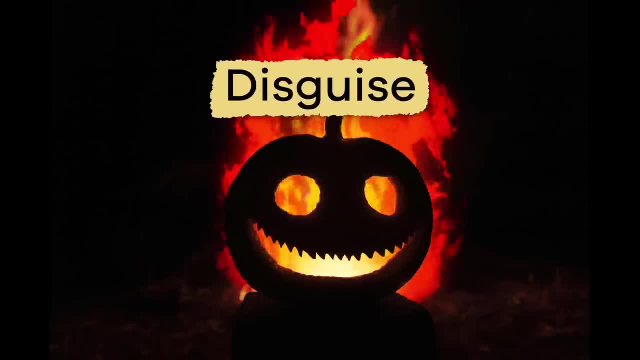 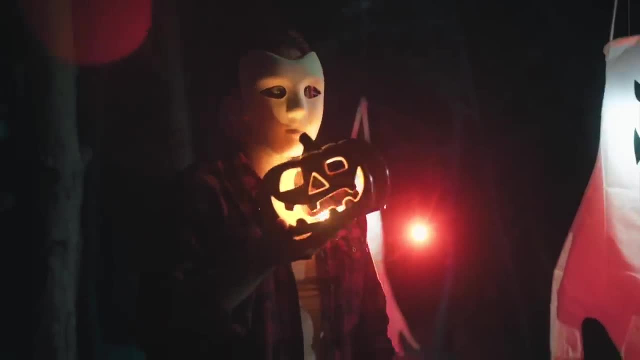 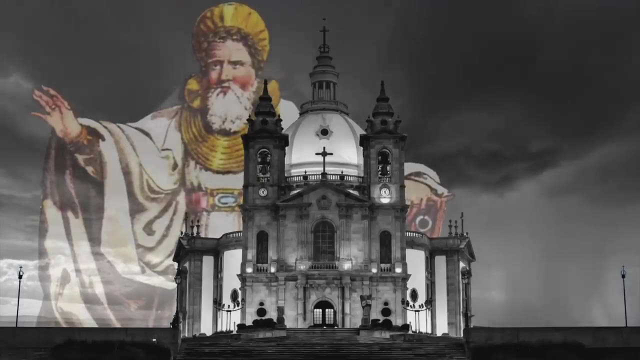 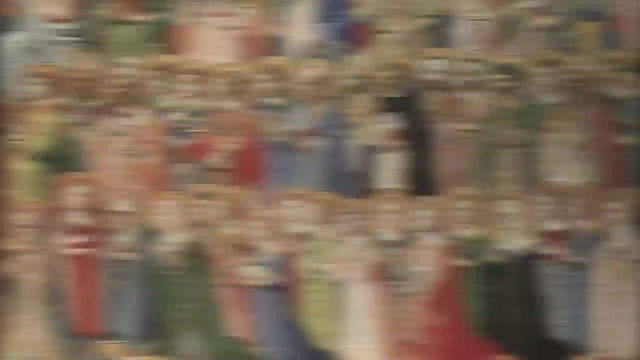 This was called guising, which is where the word disguise comes from. Are some of these things feeling a little bit familiar? Great, Let's keep learning. At the time, the Catholic Church did not recognize Celtic traditions, But in the 7th century Pope Gregory III did move a Catholic holiday called All Saints Day to November 1st. 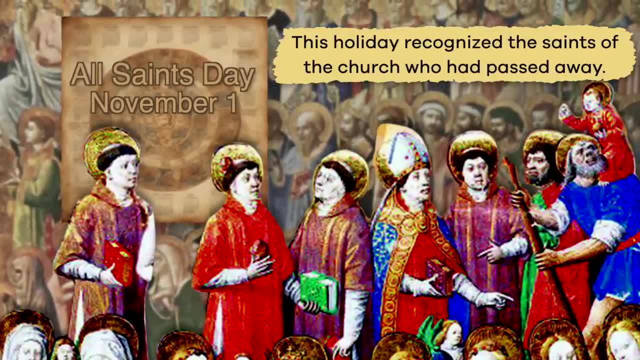 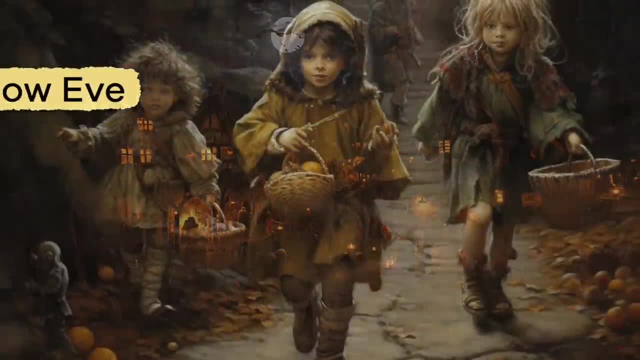 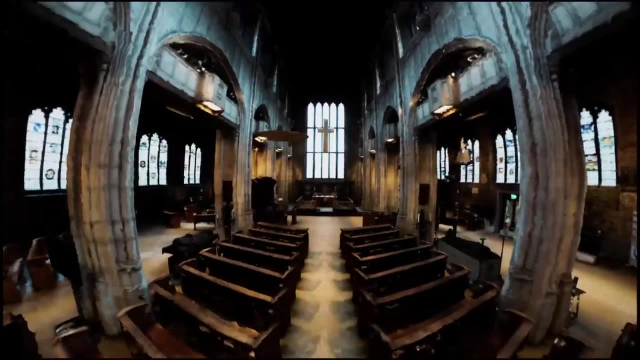 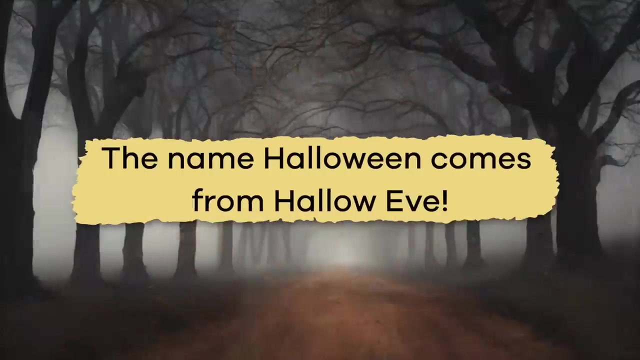 This holiday recognized the saints of the church who had passed away. Because October 31st was the day before this holiday, it became known as Hallow Eve, which then became known as All Hallows Eve. In case you were wondering, hallow is another word for holy and, as you can probably guess, the name Halloween comes from Hallow Eve. 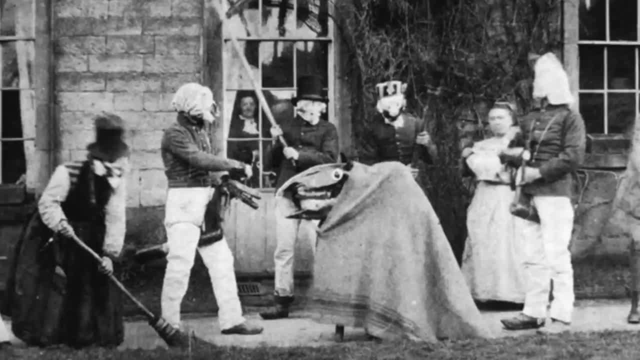 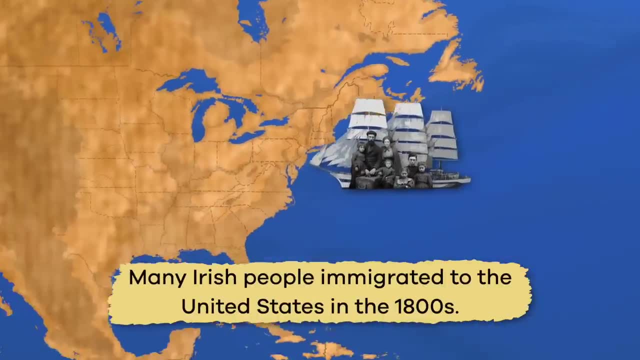 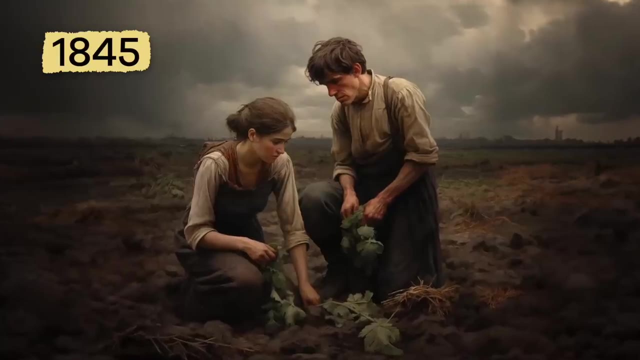 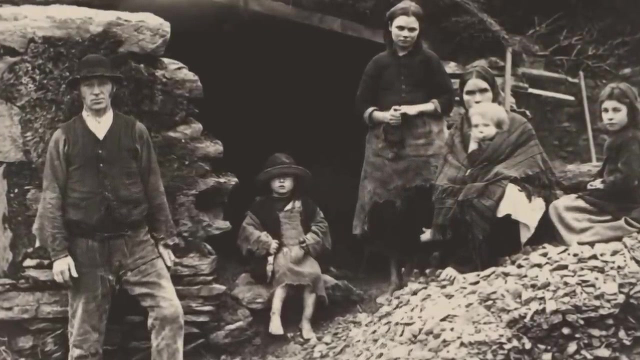 Now that we know the origins of Halloween and its name, let's talk about how it came to America. Many Irish people immigrated to the United States in the 1800s because of a tragedy called the Great Potato Famine. In 1845, a plant disease wiped out most of the potato crop in Ireland, forcing people to leave their country so they would not starve.